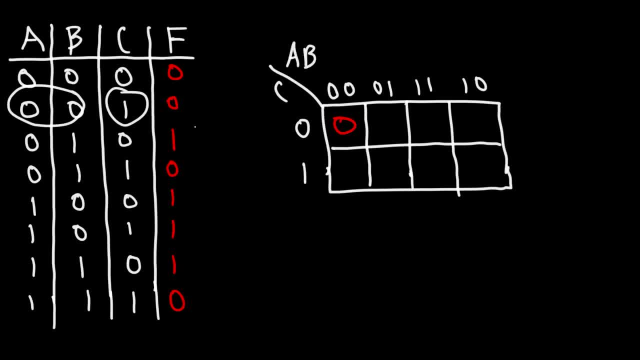 which means we're dealing with this column and c is 1,, so we're dealing with this particular square. The function value for that is still 0.. Now for the third row. we can see that a, b is 01, and c is 0, and the function value is 1, so we're going to put a: 1.. So 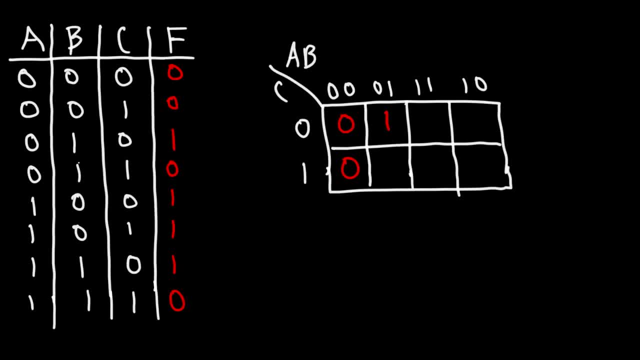 we're going to put a 1 for that square. Now for the next one, a, b is still 01, and c is 1.. So here's where a, b is 01, and c is 1, giving us this square which the function value is 0.. 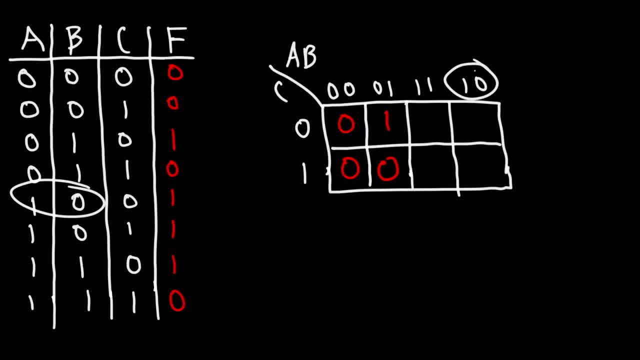 Next, a, b is 10,, so we're dealing with the last column, and c is 0,, so the function value is 1.. Now for this one: a, b is 0, and c is 1, so we're dealing with this particular square. 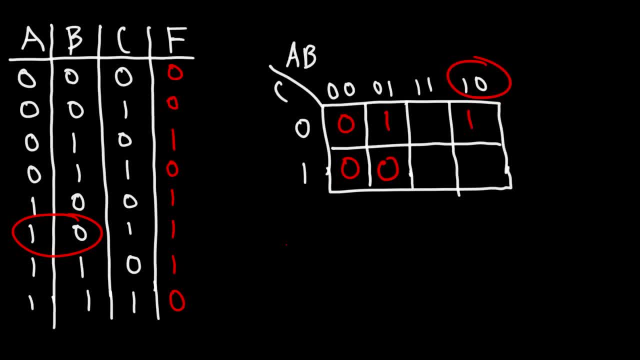 Next we have a, b is 11,, so that's the third column. c is 0, and the function value is 1.. And for the last one, the function value is 0, where a, b and c is 1.. 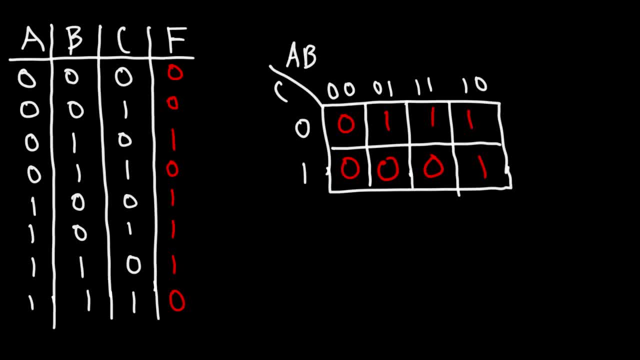 So that's how we can take the data in a truth table and put it on a column. Next, we have a cardinal map, or for short, we could say a k-map. Now how can we take this data and turn it into a function? 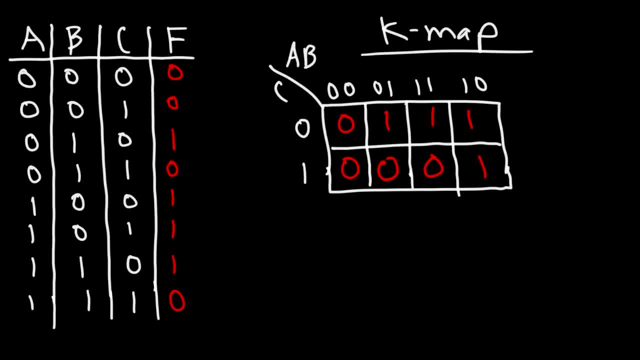 What we need to do is basically circle groups of 1s together. We can circle 1, 1,, or we could circle 2 1s, but we cannot circle 3- 1s. The number of 1s that you can circle could be 1,, 2, and 3.. 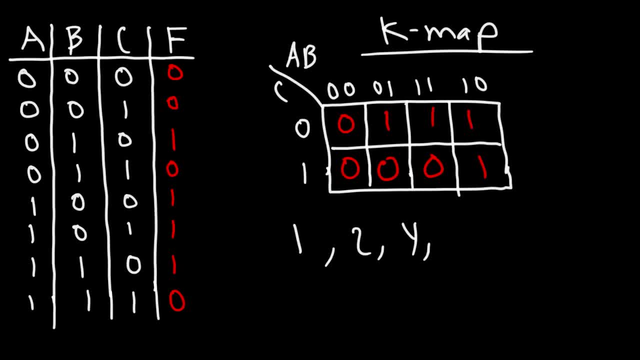 2,, 4,, 8, and so forth. It has to be a power of 2.. So you can't circle 3, 1s, 5, 1s, 6, 1s, Not going to work. 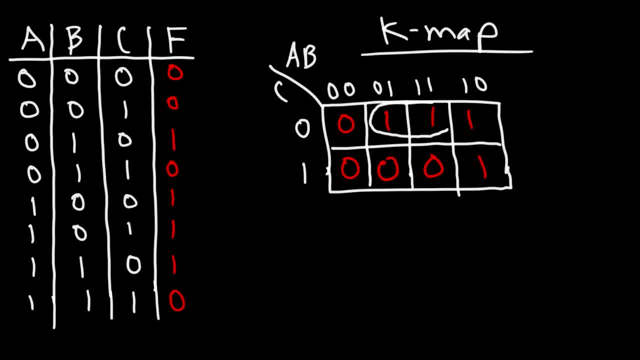 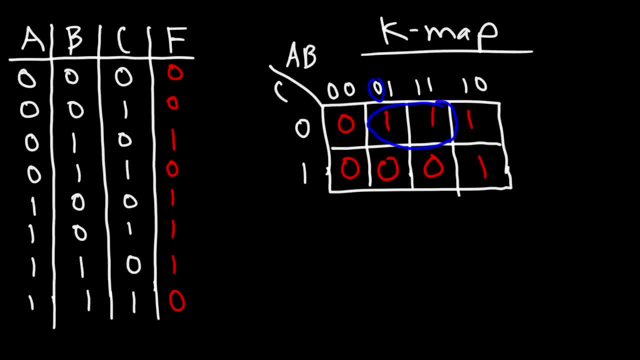 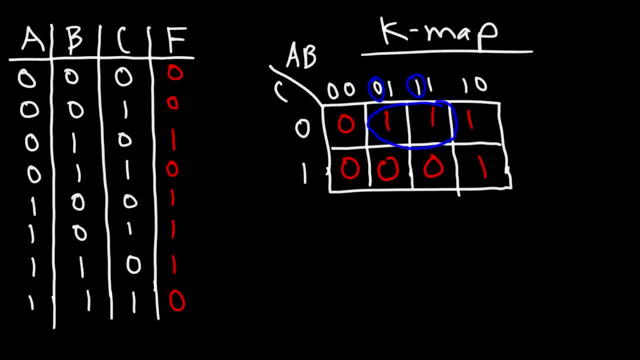 1s, 1s, 0.. 0., 1. 1s. Yet the output is the same. So the output for those two 1s doesn't depend on A. Notice that it depends on B. When B is 1, the output is 1.. 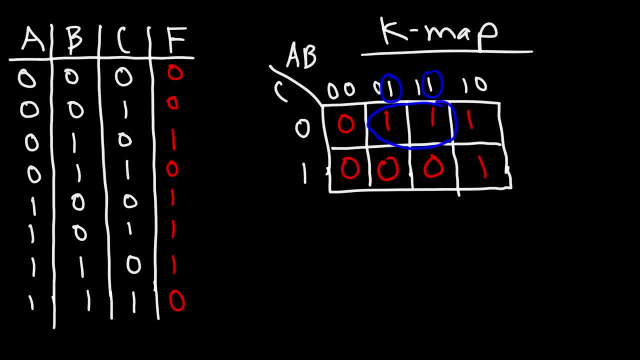 So we're looking for the variable that doesn't change. B doesn't change. So should we write B or not B? Because b is 1 and the output is 1, we're going to write b. Now these two or this pair of 1s also corresponds to a c value of 0. 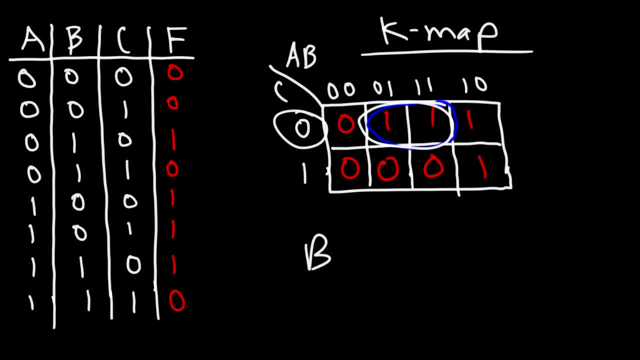 Notice that c is always 0 for that pair of 1s. So because c is 0 and the output is 1, we need to write not c. Now let's move on to the next pair of 1s. So let's put an or symbol represented by the plus sign. 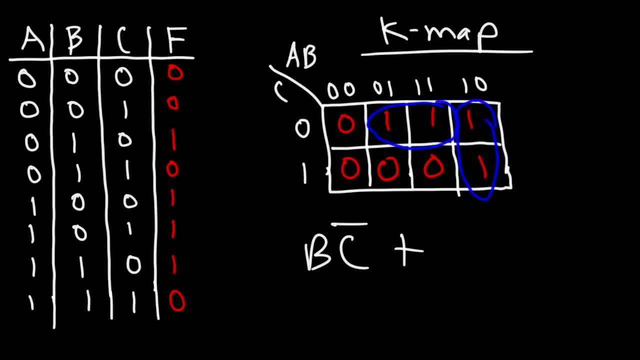 So for the second pair of 1s, what variables do not change? So notice that c changes. So for this pair of 1s, it is independent of c. But notice that ab is the same, a is 1, b is 0.. 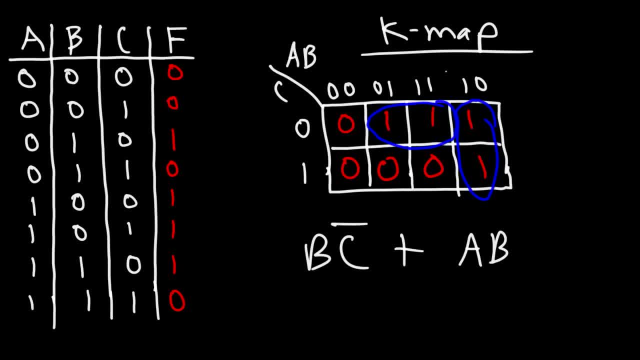 So which one is going to be? not a? Is it a or b? So because a is 1 and it matches the output function, we're going to leave it as a. But because b is 0, we need to put not b. 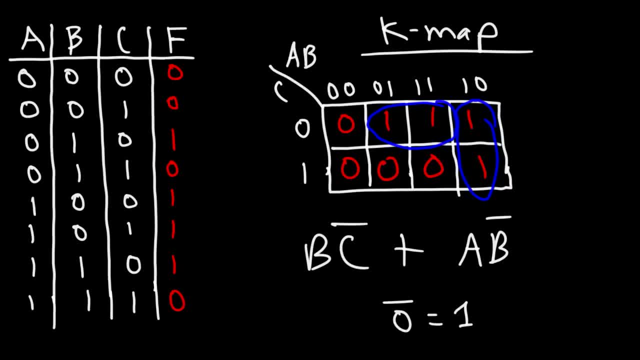 Because not 0 is 1.. So this is the function that explains this truth table. Now we can test it out. So let's see if a is 0 and if b is 1 and if c is 1, if we get a function value of 0. 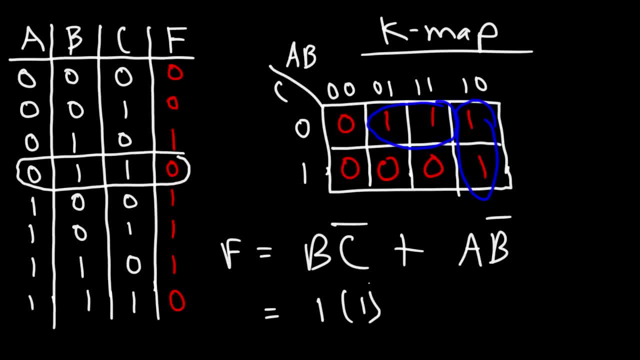 So b is 1, c is 1, a is 0, and b is 1.. So if we write the complement of 1, that's going to be 0. So we have 0 times 1, which is 0, and 0 times 0 is 0. 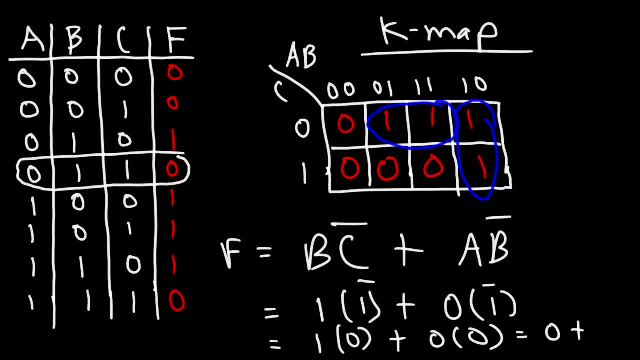 So we get an output of 0.. So that worked. Let's try another one, Let's try this one, Let's see if the function will give us the correct output. So b is 0, c is 1, a is 1, and b is 0. 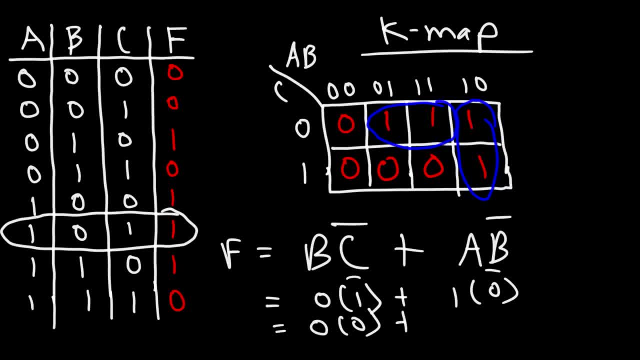 Now the complement of 1 is 0, and the complement of 0 is 1.. 0 times 0 is 0,. 1 times 1 is 1.. 0 plus 1 is 1.. So we get the right output. 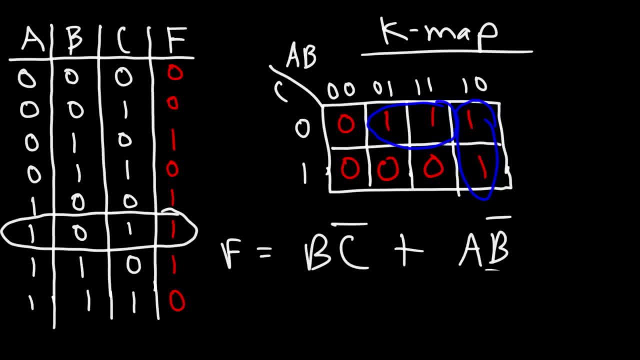 Now, for the sake of practice, let's make sure that we have the right function. Let's try the last one. So b is 1,, c is 1, a is 1, and b is 1 as well. So the complement of 1 is 0.. 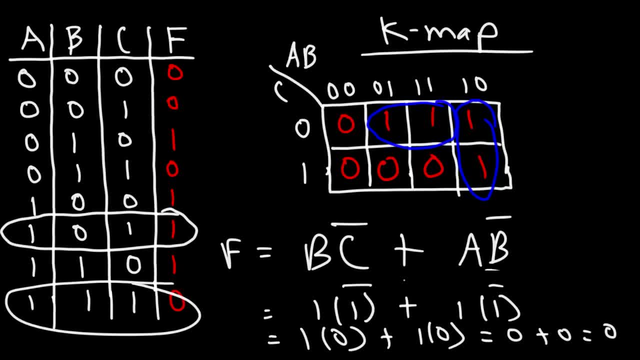 And 1 times 0 is 0.. 0 plus 0 is 0. And we can see that we have the correct output. So we have the correct function. So that's how you could use a carnal map to quickly write a function that corresponds to a truth table. 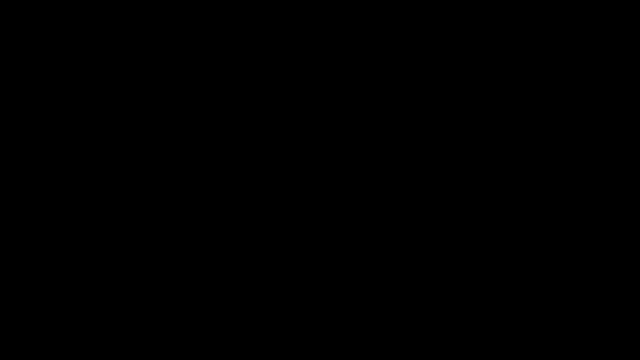 Now let's take the function that we have and turn it into a circuit diagram. So the function that we have was b times the complement of c plus a times the complement of b, So we can write that as b c prime plus a b prime. 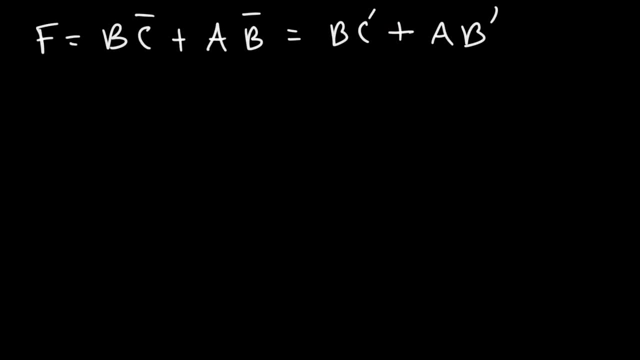 So we need an AND gate to connect b and c prime. So let's start with that. And we need another AND gate to connect a and b prime. So this is going to be b and c prime, And here we have a and b prime. 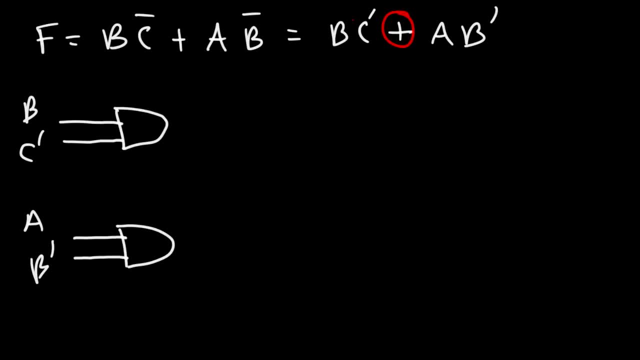 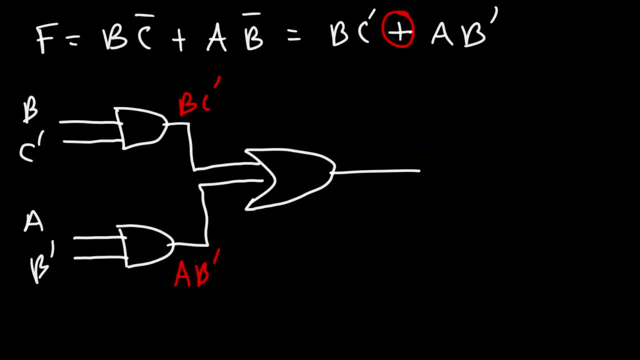 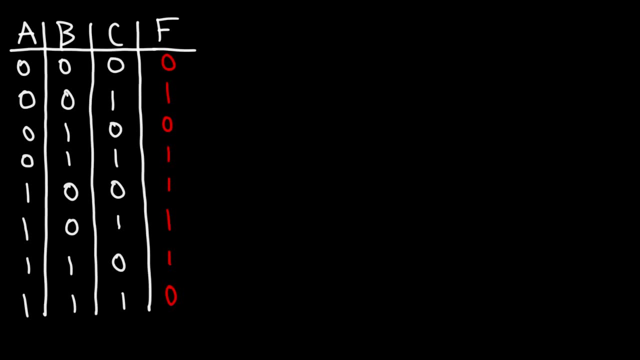 And the output of the OR gate is going to give us the function f, which is what we have here. So that's the circuit diagram that corresponds to this function. Let's try another example. Let's use this truth table to create a k-map and then use that to write a function. 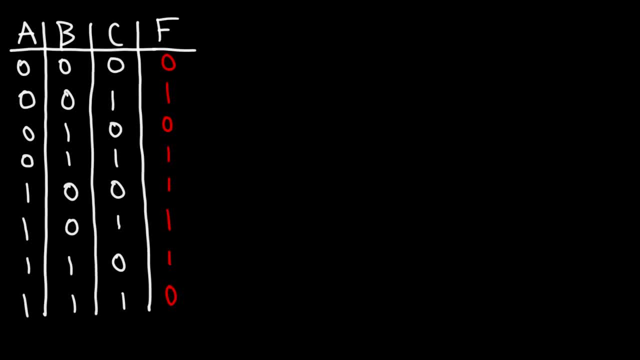 which will then use that to turn it into a circuit diagram. If you want to pause the video and try this problem, feel free. Now, the type of k-map that I'm going to draw is going to be a little bit different than the last one. 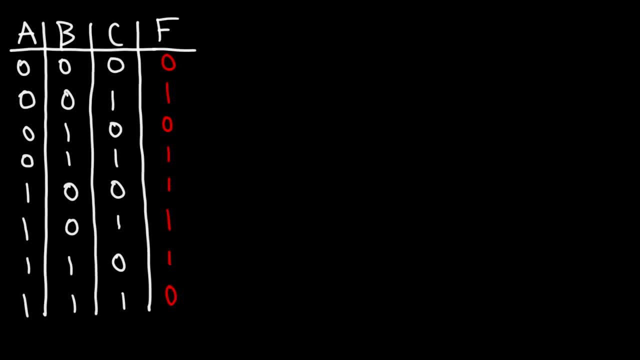 The last one was a three-variable k-map drawn in the horizontal direction, But I'm going to draw one with a vertical orientation. So instead of having two rows, four columns, I'm going to have two columns, four columns, four columns, four columns. 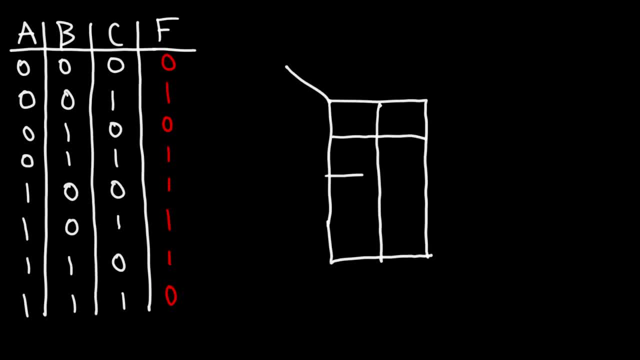 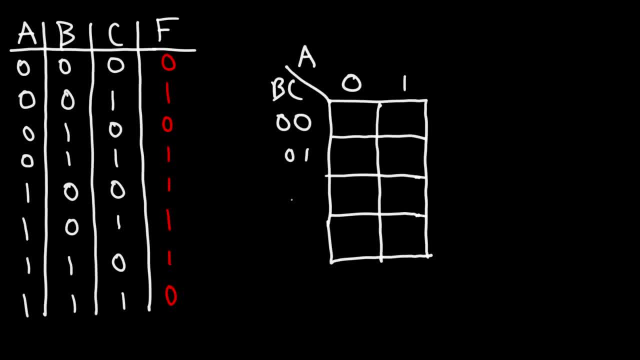 bc can be 00,, 01,, 11, or 10.. So that's how you can draw a three-variable k-map with vertical orientation. Now let's fill in a table. So for this first column, a is 0,, which we can see it for the first four inputs. 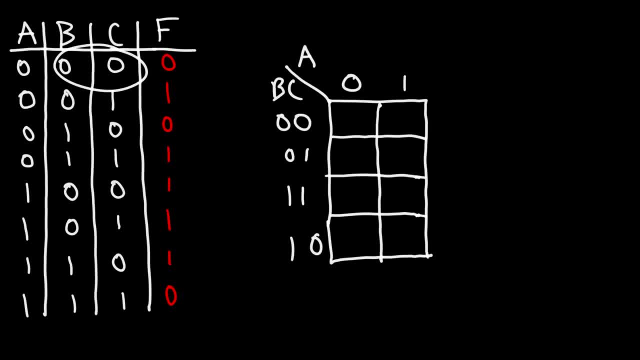 So here, when b and c is 0,, the function is going to be 0.. And when bc is 01,, the function is going to be 1.. When bc is 10,, the function is 0.. And when bc is 1,. 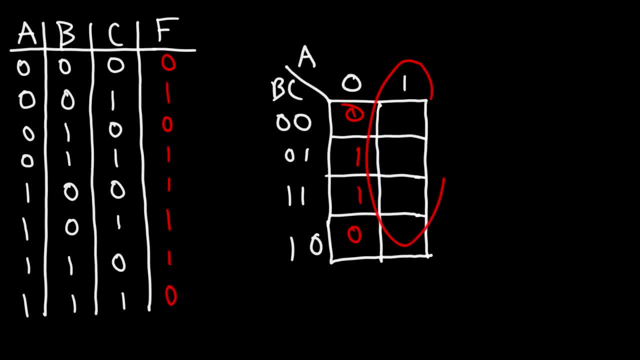 the function is 1.. Now for the second column, a is always 1,, which will correspond to these four. So when bc is 0,, the function is 1.. And when bc is 01,, the function is also 1.. 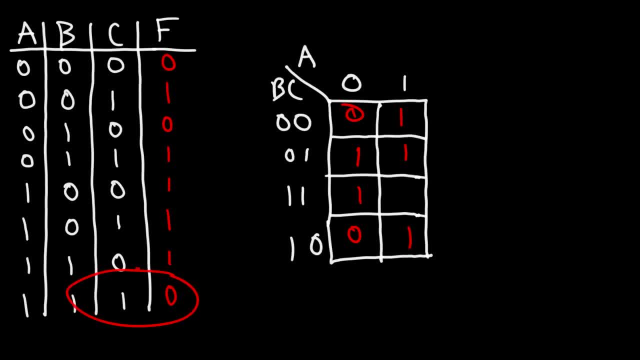 When bc is 10,, the function is 1.. And when bc is 11,, the function is 0.. So that's how we can quickly fill out this k-map. Now, how can we use it To write a function for the truth table? 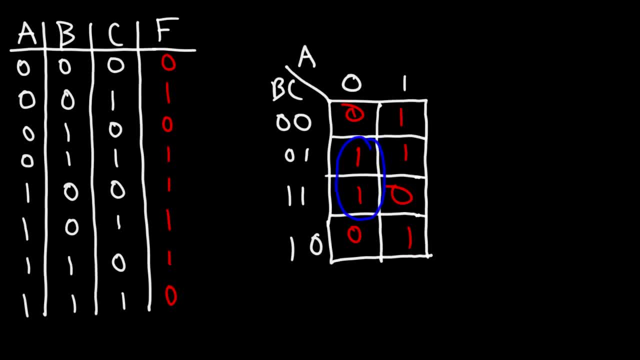 So let's start with this pair of 1s. Notice that a is always 0. So we need to write the complement of a, Because the complement of 0 will give us an output of 1.. Now for those pair of 1s. notice that b changes. 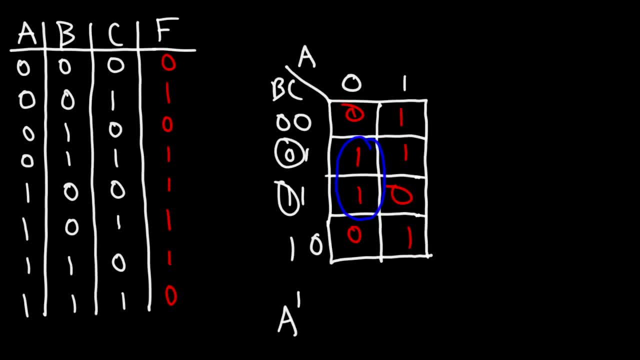 So the output is independent of b. So we're not going to include b, But notice that c is 1.. So we're just going to write c. Now let's draw the next pair of 1s. So notice that a is always 1 for that group. 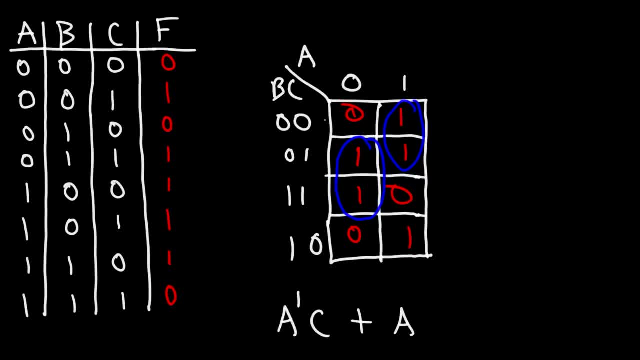 And this time c changes, So it's independent of c, But b is consistent: b is always 0. So we're going to write b'. Now there's only one last one that we need to consider, And that's here. 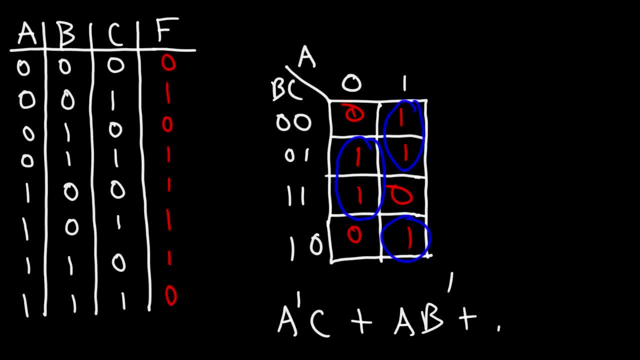 So a is 1.. We're just going to write a. b is 1.. We're going to write b And because c is 0, we're going to write c' So this is the function that corresponds to this truth table. 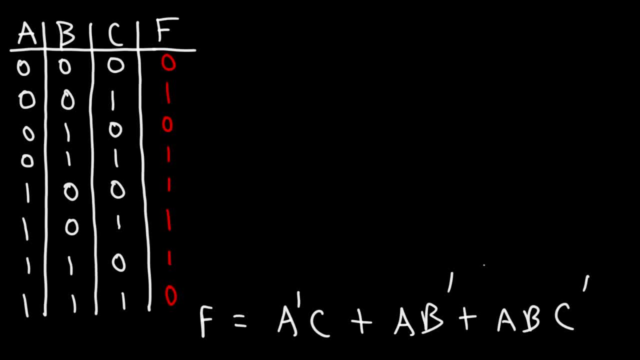 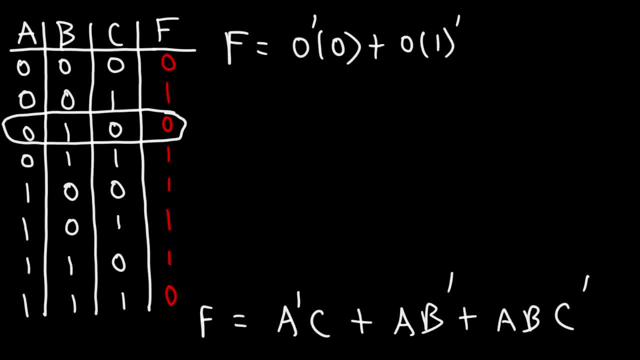 a is still 0.. b prime b is 1.. And then we have a b- c prime. So a is 0.. b is 1.. c is 0.. The complement of 0 is 1.. The complement of 1 is 0.. 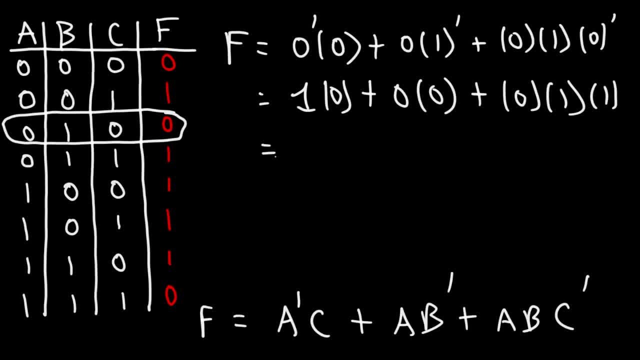 And the complement of 0 is 1.. 1 times 0 is 0.. 0 times 0 is 0. And 0 times 1 is also 0. So this adds up to 0, which we can see. that's the case. 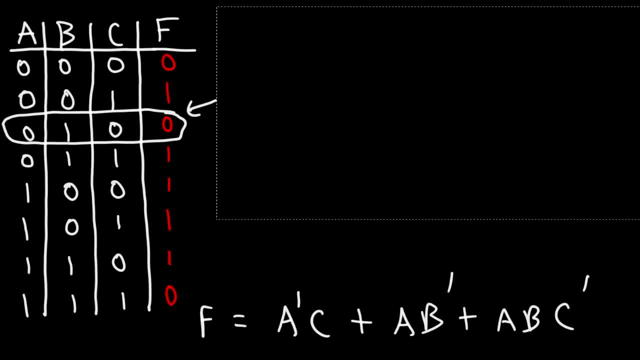 Now let's try one more. Let's try this one where a, b and c is a, 1. So we have the complement of 1 times 1 plus 1 times the complement of 1 plus 1 times 1 times the complement of 1.. 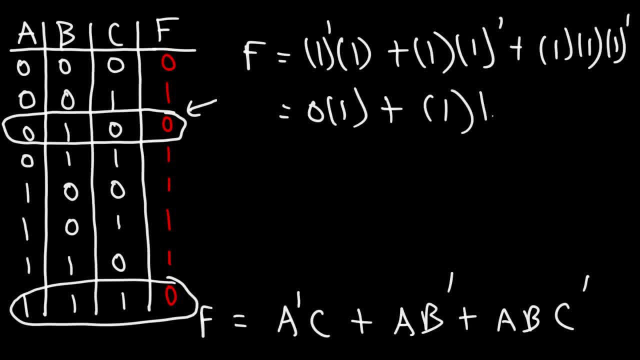 The complement of 1 is 0. So automatically, 0 times 1 is 0.. 1 times 0 is still 0. And the last one is going to be 0. So the output is once again 0.. 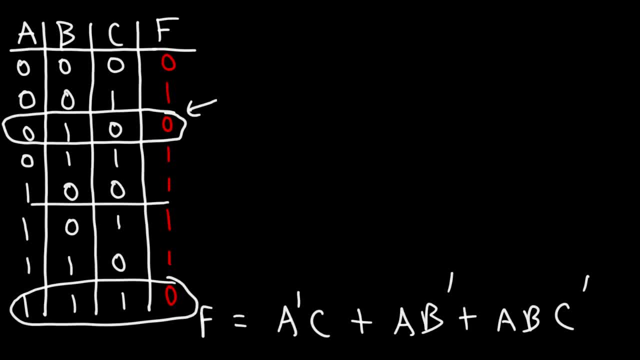 Okay, let's try one that's going to give us a value of 1.. Let's try this one. So a is 1.. c is 1.. b is 0.. And a is 1.. b is 0.. 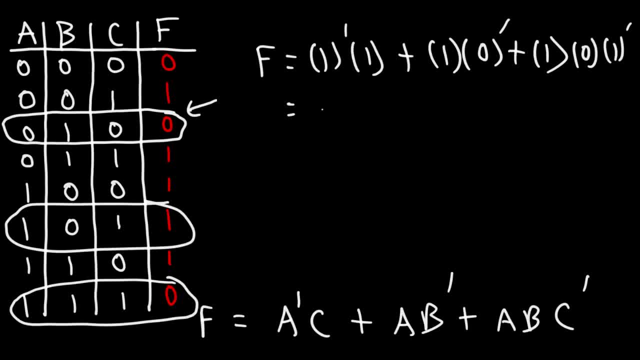 c is 1.. So the complement of 1 is 0.. The complement of 0 is 1.. And the complement of 1 is 0.. 0 times 1 is 0.. 1 times 1 is 1.. 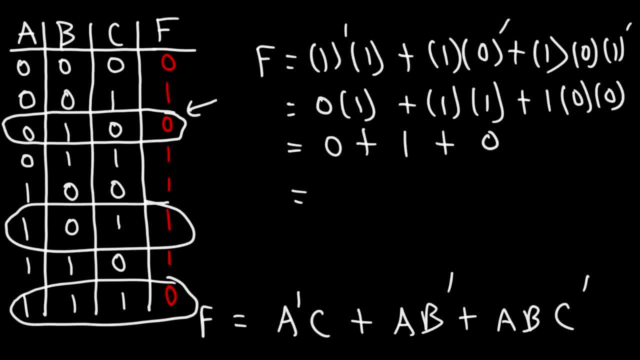 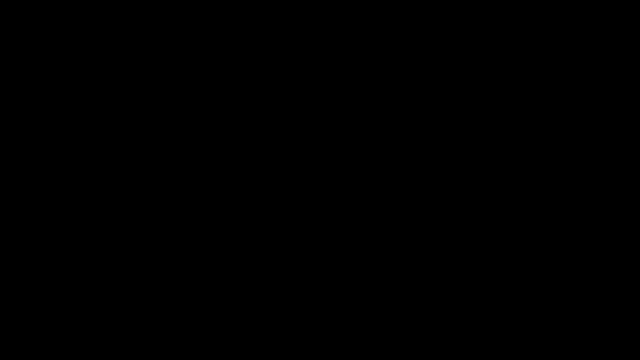 1 times 0 times 0 is 0.. 0 plus 1 plus 0 is 1.. So this function works. So now you know how to write a function using the KMAP. but now let's turn this function into a circuit diagram. 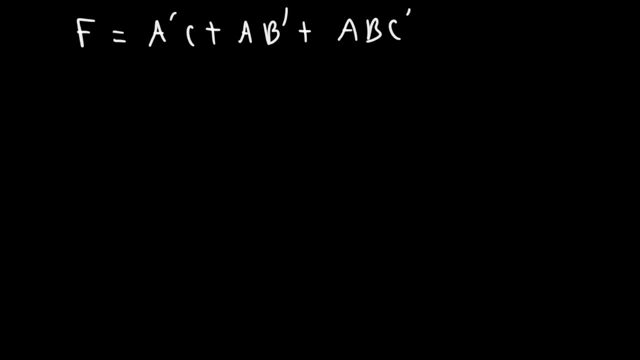 Let's draw the logic circuit that corresponds to this function. So let's start with the first term that we have. So we need an AND gate, So it's going to be A prime C and the output will be A prime C. Now for the second AND. 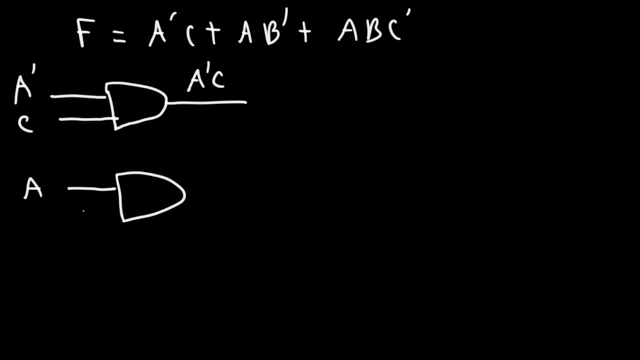 gate. the input will be A and the second input is going to be B prime, giving us the output A, B prime. Now for the last one, I'm going to use a three-input AND gate, So the three inputs will be A, B and C prime. 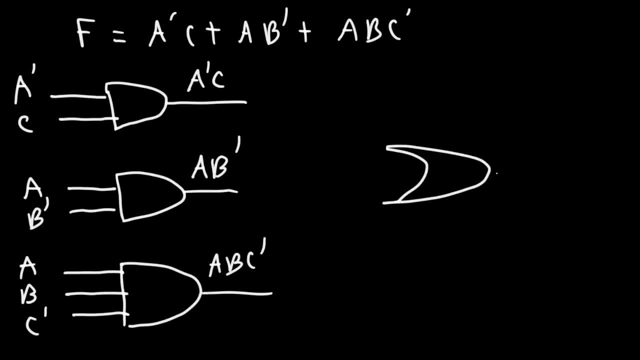 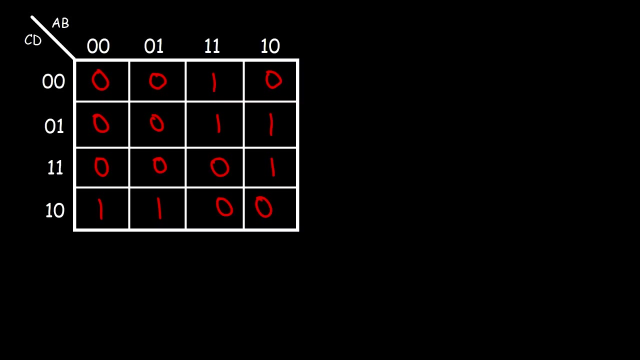 Now we need a three-input OR gate. Then this will give us the output function F, And so that's how you can draw the logic circuit for this particular function. Consider the four-variable KMAP that we have on the screen. Go ahead and write a function for this KMAP. 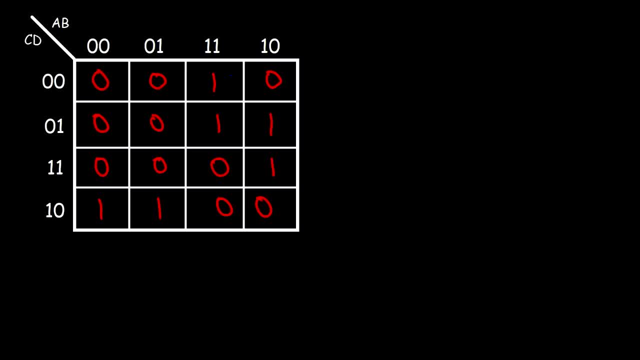 Feel free to pause the video. So first let's begin by analyzing those two pair of ones. So notice that A and B is always one for that selection. So we have A and B And for that selection, notice that C is always zero but D changes. 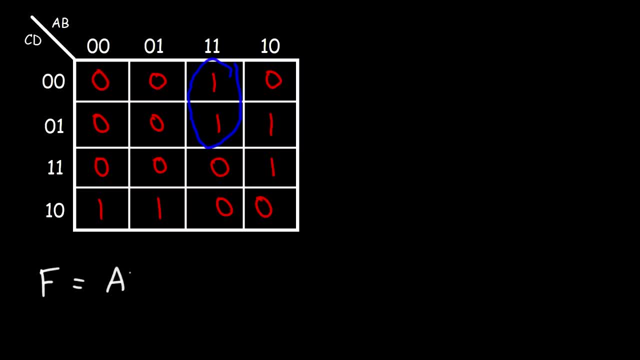 So it depends on C, but not D. So we have A, B, and since C is zero, we're going to have C prime. Now let's select another pair of ones, So let's go with that. Now notice that A is always zero. 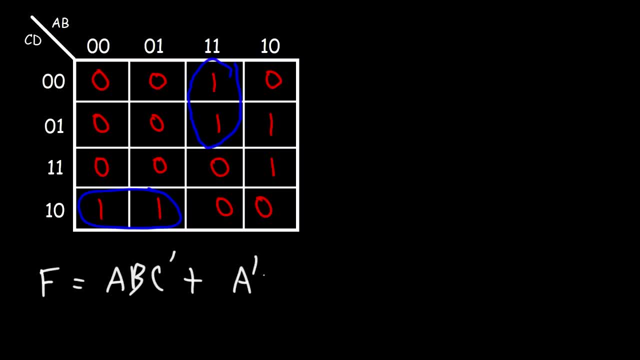 So we're going to have A prime. B changes, so it's going to be independent of B. Now, C is always one and D is always zero, So we're going to write D prime. Now let's select this pair of ones that we have there. 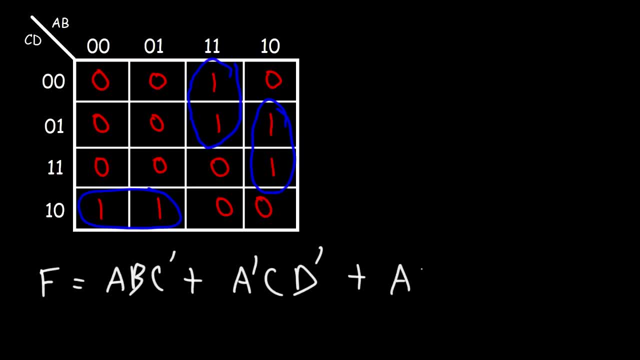 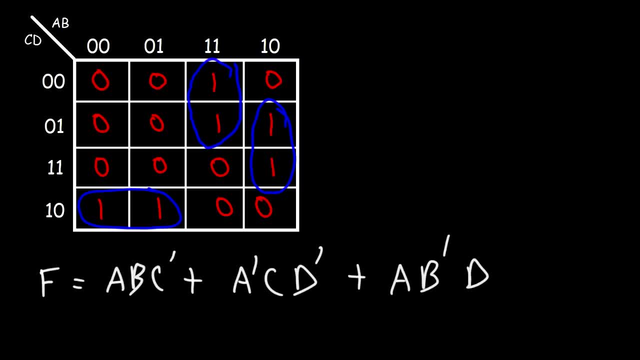 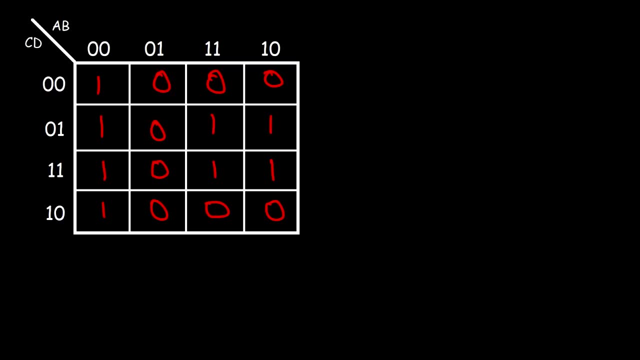 D is always one. So this is going to be A, B, prime D. So this is the function that corresponds to this particular four variable K-map. Let's try another example. Go ahead and try this one. So, instead of selecting two 1s, we can select a group of four 1s. 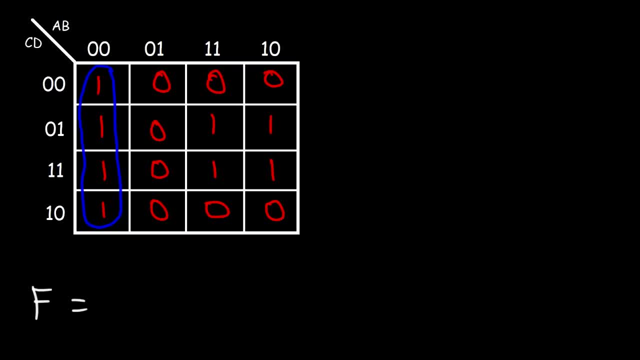 So for that particular group, which variables remain the same. Notice that a is always 0 and b is always 0. So we're going to have a prime and b prime. Now c can be 0 or 1, so it's independent of c. 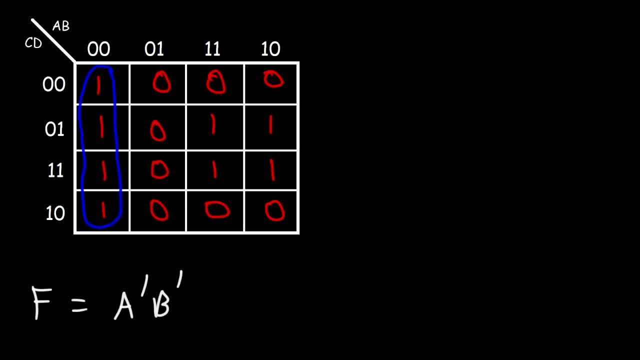 And d can also be 0 or 1.. So it's only going to depend on a and b for that first selection. Now the next selection: we can basically take a square of 1s, So which variables are constant. Notice that a is always 1.. 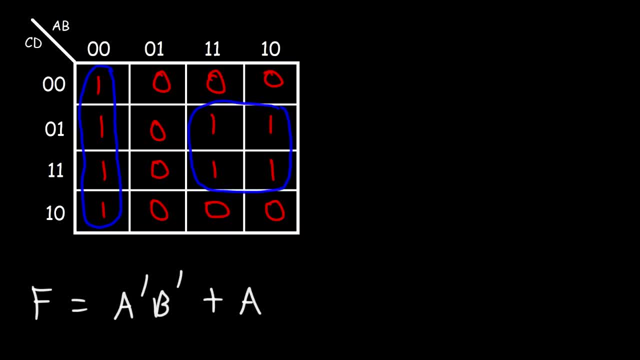 So we're going to write a. b changes between 1 and 0, so it's independent of b. On this side, notice that d is always 1.. So it's going to depend on d. c changes, So it's independent of c. 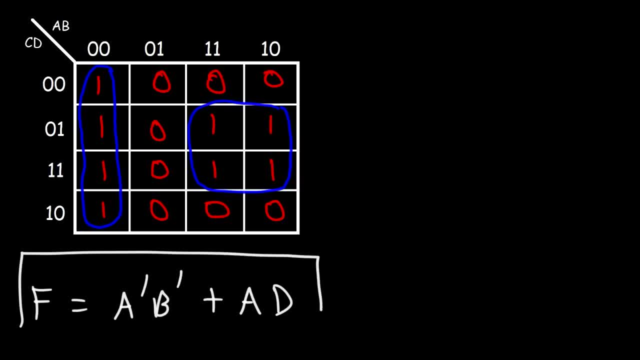 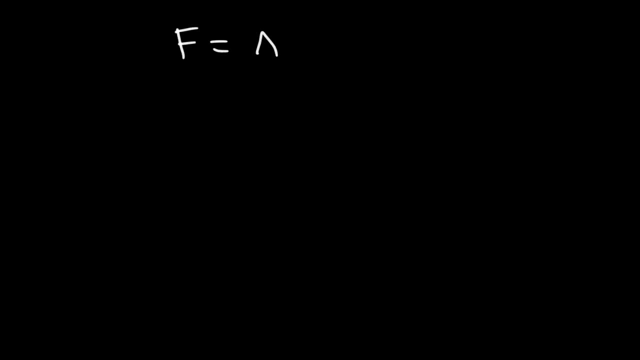 So this particular function is represented by this equation. It's a prime b prime plus a d. So now you know how to take the information from a four variable k-map and turn it into a function. Now let's say that we're given a function: a c plus a b prime. 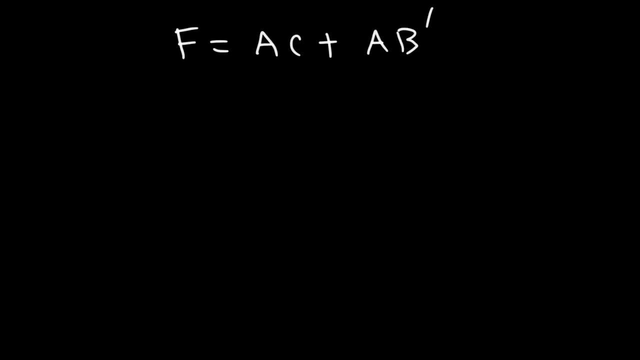 So how can we take this function and create a three variable k-map? And let's create it in a horizontal direction, So we're going to need two rows and four columns. So we're going to put a, b above the diagonal line and c below it. 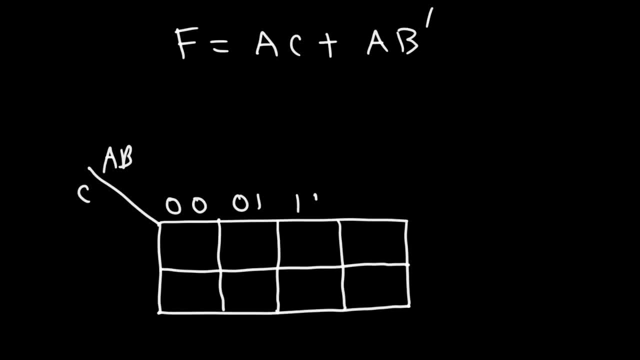 So a, b can be 0, 0,, 0, 1,, 1, 1, or 1: 0. And c could be 0 or 1.. Now let's focus on the a- c term. Notice that we don't have any complements here. 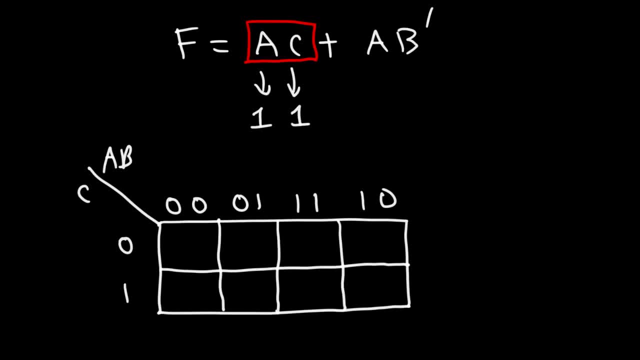 So we're looking for when a is 1 and when c is 1.. c is 1 anywhere in this row. a is 1 here. So what we're going to do is we're going to put a 1 in those boxes. 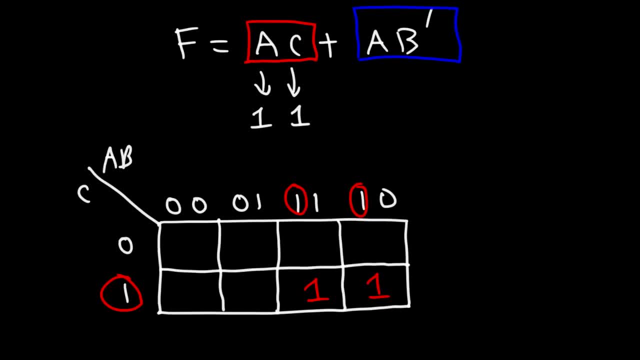 Now let's focus on the next term: a, b prime. So we just have a, we're going to put 1.. We have the complement of b, so we're going to write 0.. So let's identify where a is 1 and b is 0.. 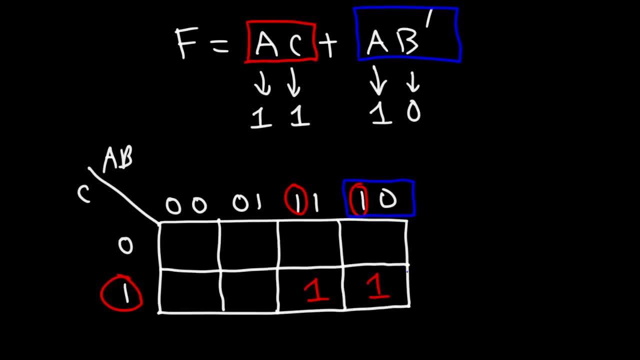 So this is when a is 1 and b is 0.. So anywhere in this region. So we need to fill this row with a 1.. And we have an overlapping 1 there. Now every other box we're going to put a 0 in it. 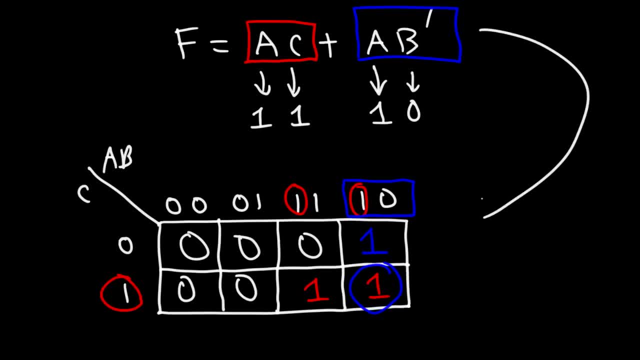 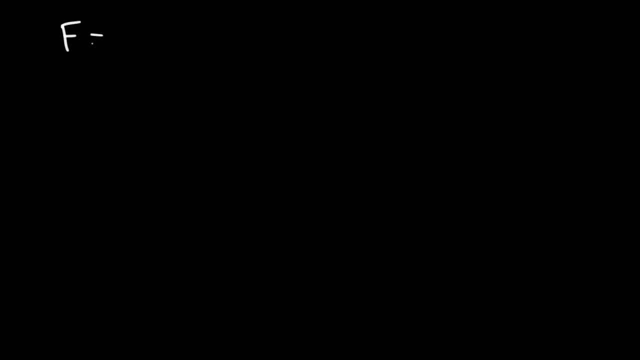 So that's how we can take a function and draw a k-map from it. Now let's try another example. So let's say the function is a b prime plus a c plus a prime, b, c, prime. So let's create another three variable k-map, but in the vertical orientation. 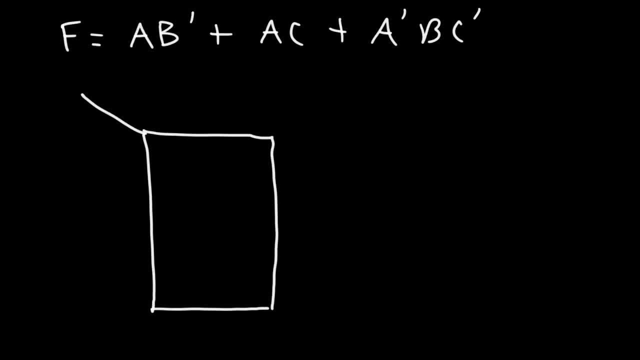 So we're going to have two columns and four rows, So we're going to put the letter a on top, b c below the diagonal line, So a can be 0 or 1, b, c can be 0, 0,, 0, 1, 1, 1 or 1, 0.. 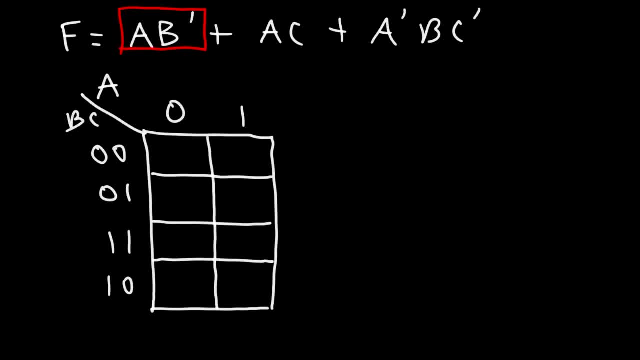 Now let's start with this term: a, b prime. So a is going to be 1.. b is going to be 0.. a is 1 in this column, So let me just highlight that in red And b is 0 here. 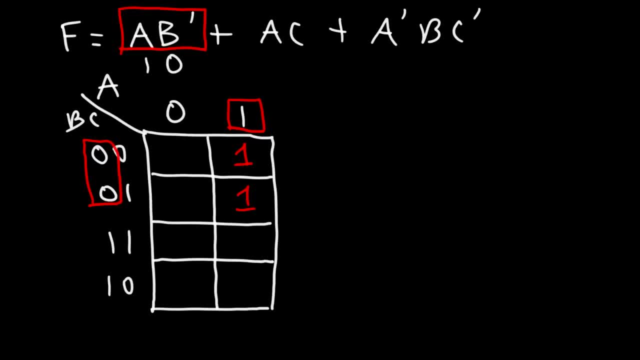 So that means we're going to put a 1 in those first two boxes on the right. Now let's move on to the next term, a, c. So that's when a is 1 and when c is 1.. So we need to put a 1 in here. 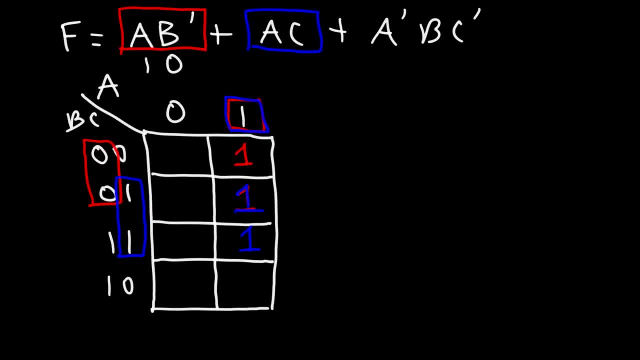 We need to put a 1 here and here. Now for the next one. we have a prime, b, c prime. I forgot to put 1: 1 for that. Now, for a prime, we're going to write 0.. For b, we're going to put 1.. 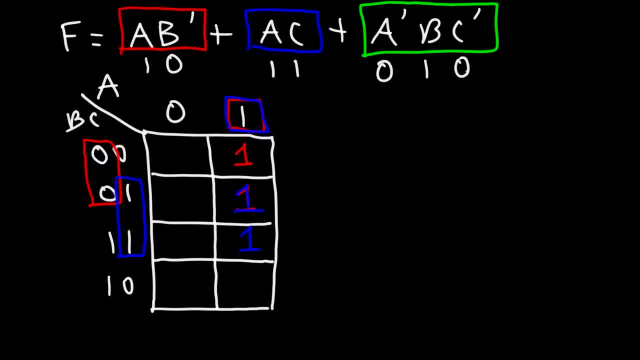 For c prime we're going to write 0. So a is 0 in the first column And b is 1.. So we need to put a 1 in here And c is 0 here. So we want a to be 0 and b to be 1 and c to be 0.. 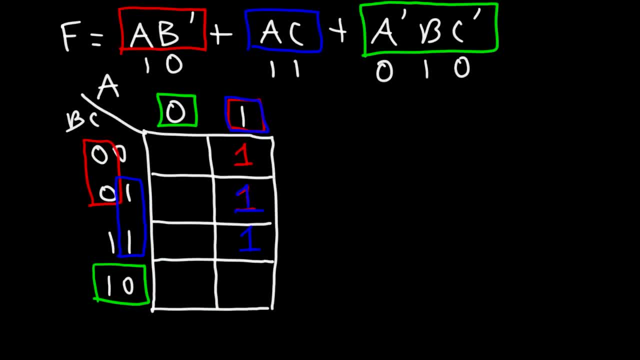 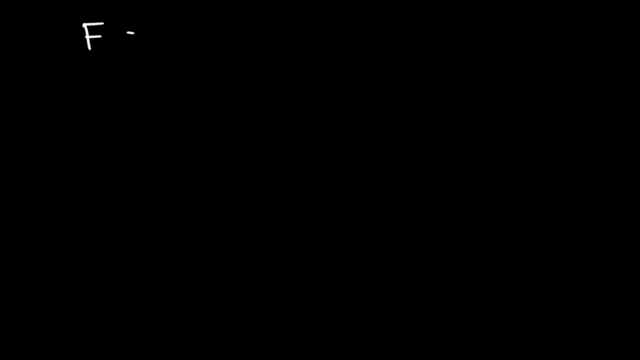 So that only corresponds to this last square. So we're going to put a 1 there. So every other box, we're going to put a 0. And so that is the k-map that corresponds to that function. Here's another, harder example. 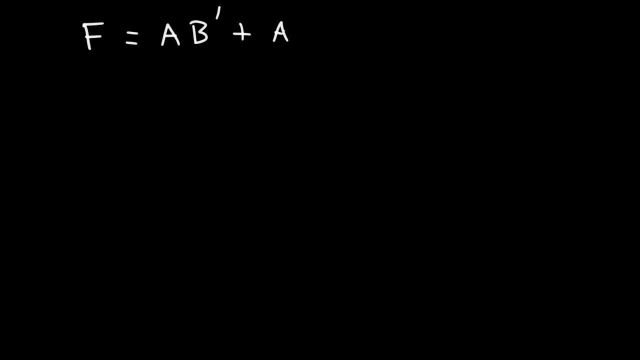 Let's say the function is 0. The function is a b prime plus a prime, c d plus a b c prime. Go ahead and draw a k-map for that function. Now, what type of k-map do we need? 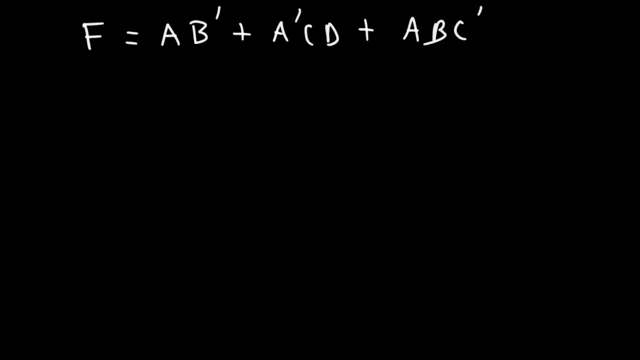 Would you say it's a 3-variable k-map or a 4-variable k-map? Notice that we have 4 variables: a, b, c and d. So this time we're going to need 4 columns and 4 rows. 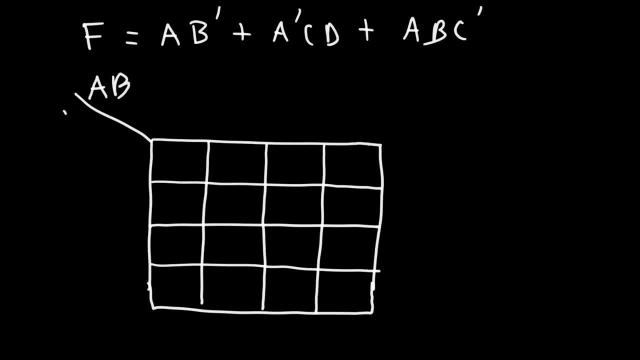 So let's put the letters a- b on top and c d on the bottom, So a? b could be 0, 0, 0, 1, 1, 1, and 1, 0.. And the same is true for c d. 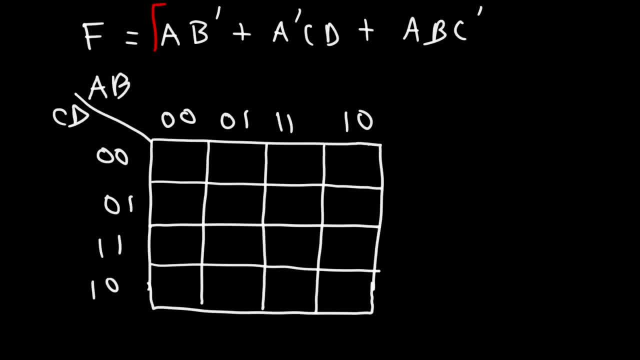 Now let's focus on a b prime. So we have a, which we're going to put a 1 for that, And for the complement of b, let's put a 0. So when is a 1 and when is b 0?? 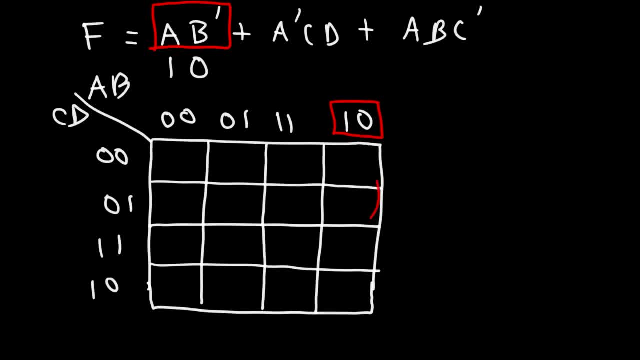 a is 1 and b is 0 anywhere in this column. So we're going to put a: 1 everywhere in that column. Now let's move on to the next term. We're going to put a: 1 for a and b and a- 0 for the complement of c. 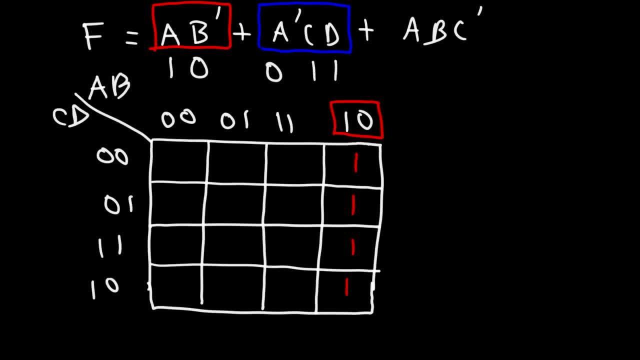 So let's put the 0 for the complement of a and a 1 for c and d. So notice that c and d is 1 in this region And a is 0 in the first two columns. So therefore we have to put a 1 at the intersecting squares. 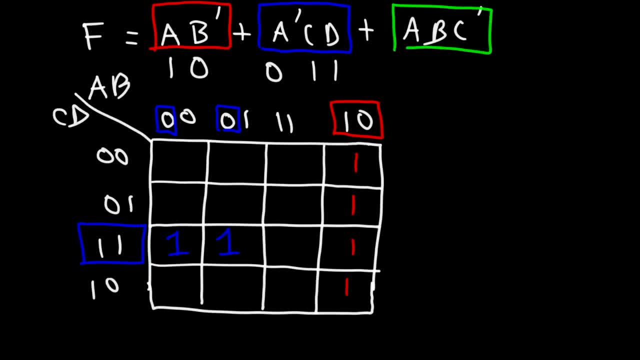 Now for the last term: a, b, c prime. We're going to put a: 1 for a and b and a: 0 for the complement of c. So a and b are 1 in this region. c is 0 in the first two rows. 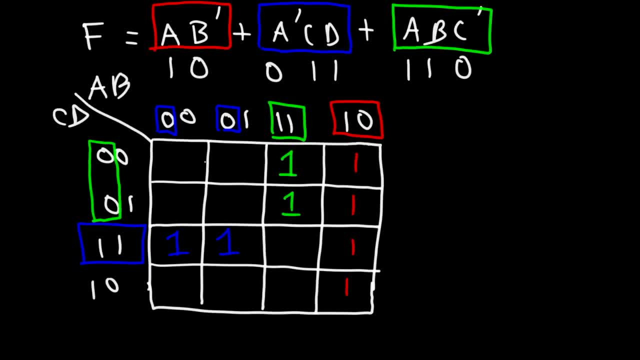 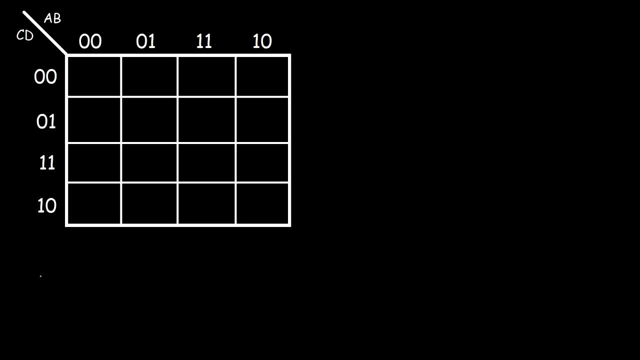 So we're going to put a 1 here. Everywhere else we're going to fill it in with a 0.. And so now we've completed the four-variable k-map, Let's work on one more example. So this one I'm going to color code differently. 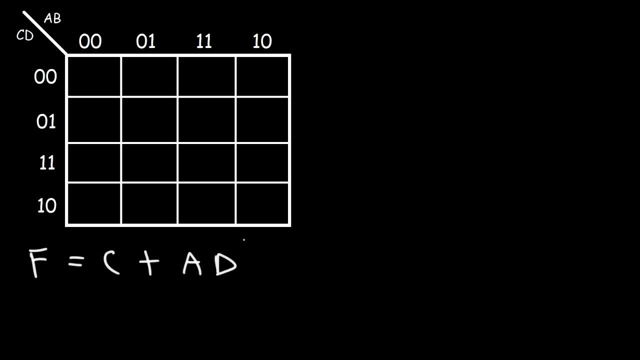 So let's say the function is c, a, d prime plus a prime, b, c, prime d plus a, b prime c. So go ahead and fill out the four-variable k-map given this function. So let's start with the letter c. 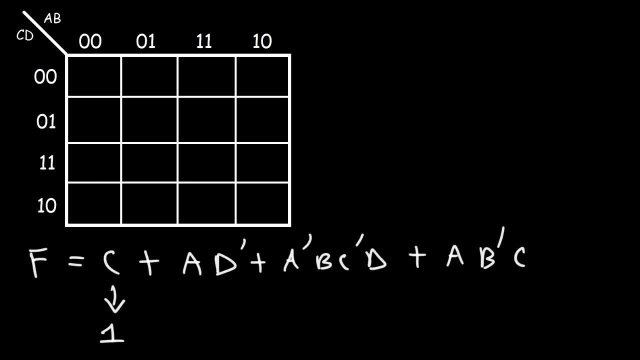 So since we have c and not the complement of c, it's just going to be 1.. c is 1 in this region, So that's anywhere in the last two rows. So we're going to have to put a 1 in all of those rows. 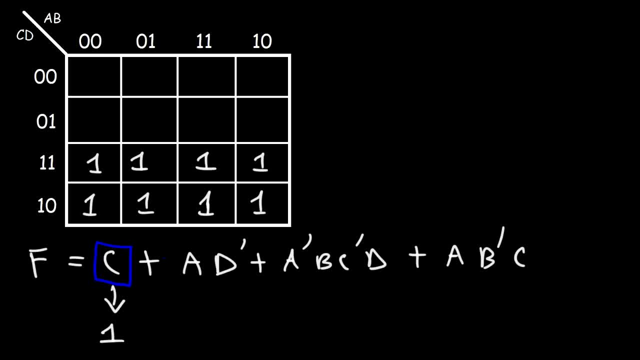 I mean in those two rows. So I'm going to color code this group of eight 1s. Notice that when we have just a term with one variable, we're going to get eight 1s. For a term with two variables, we're going to get four 1s. 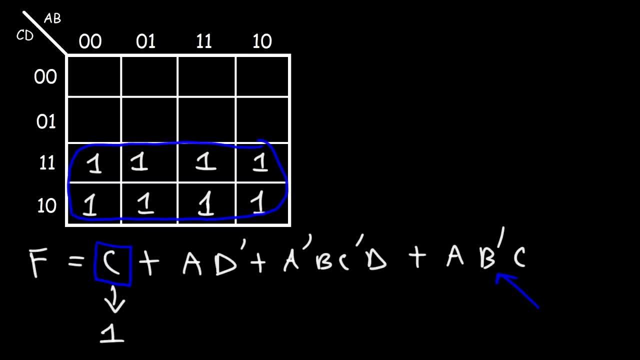 For a term with three variables, we're going to get two 1s, And for a term with four variables, we're only going to get one 1.. So let's move on to the next one, a d prime. So for a, I'm going to put 1.. 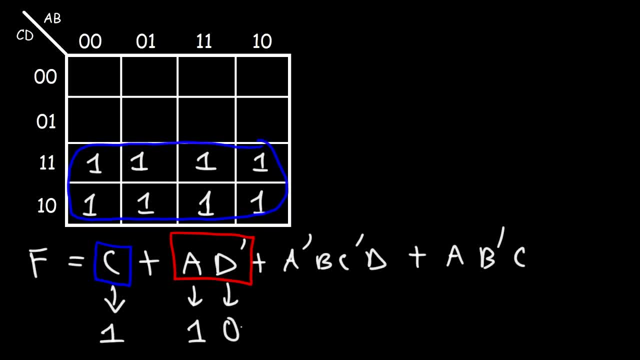 And for d prime 0. So a is 1 in the last two columns on the right And d is 0 here. So we're going to have a 1 and d's as well. So now I'm going to circle those 1s with a red color. 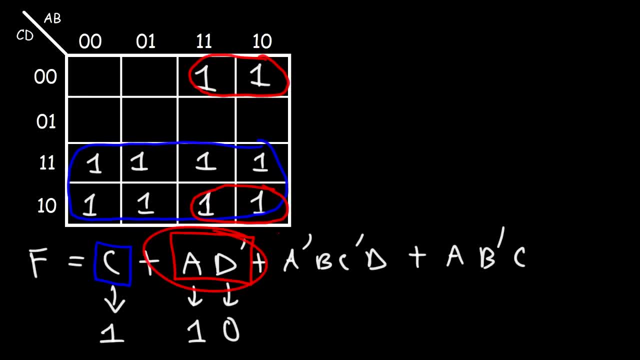 So, as we can see, for a term with two variables, we have a total of four 1s highlighted in red. Now let's move on to the next term, Which has four variables. So we should only get one 1 in the K-map. 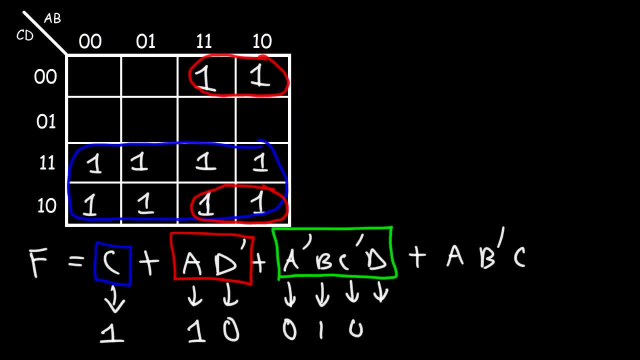 So for a prime we're going to write 0.. For b: 1. c prime: 0.. d: 1.. So a is 0 and b is 1 here, c is 0 and d is 1 here. 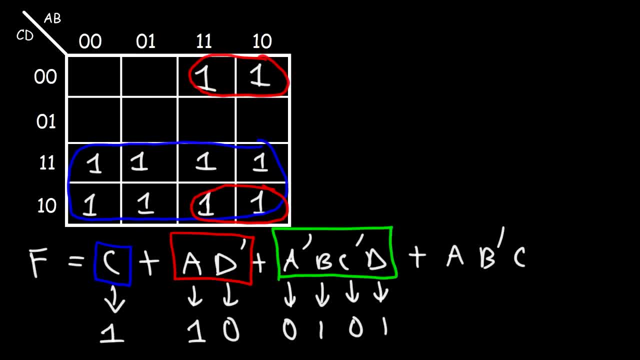 So we're just going to put a 1 in this region And I'm going to highlight it in green. Now for the last one: a b, prime, c. So we're going to have a 1 for a, 0 for b prime and a 1 for c. 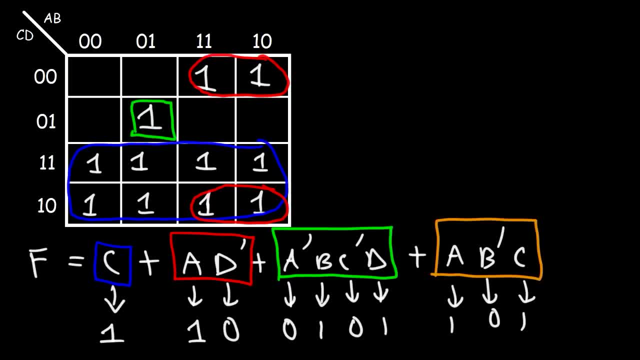 So first let's identify where a, b is 1, 0.. So that's going to be in this region. And now let's identify where c is 1.. c is 1.. In the second and the third row from the top. 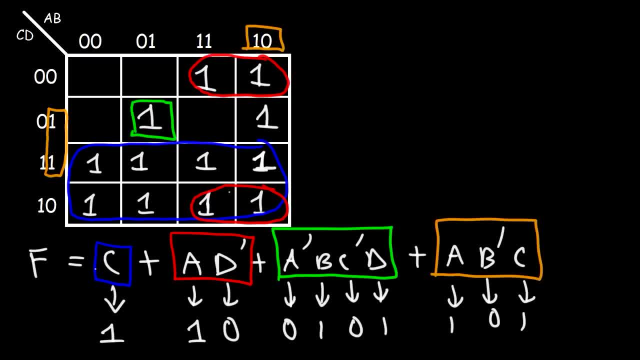 So we're going to need a 1 here and the one that we already have here. So, as you can see, for a term with three variables we get a pair of 1s or two 1s. Everything else let's put a 0..